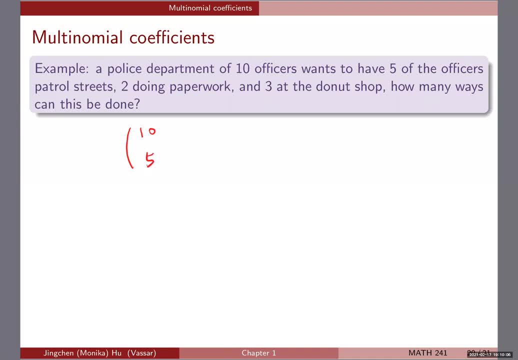 well is a choose function can choose five. okay, So we're done with that. And the next step? well is, once we have chosen the five, we have five remaining officers to patrol the street. okay, So that, well is a choose function, can choose. 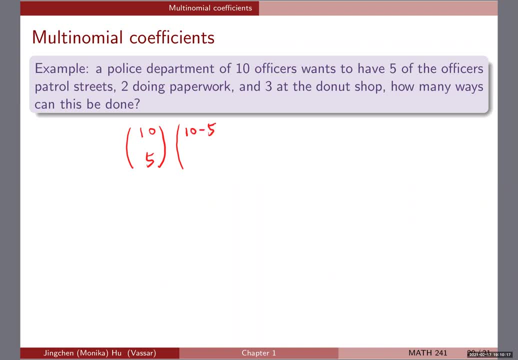 remaining right. So if we want to write it, it's 10 minus five, and we are choosing two of them to do the paperwork, okay, And the last one. well, we know that we have remaining to five minus two. 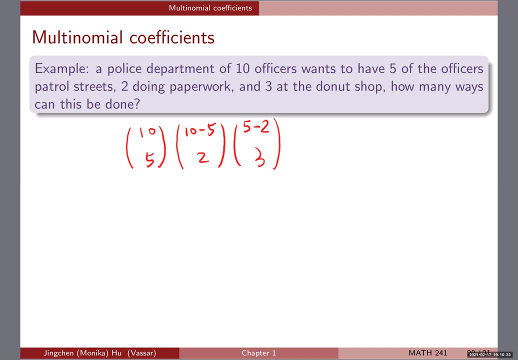 and all of them will be at the donut shop, right? So, to write it more completely, this is what we do, but then we can quickly reduce this into 10: choose five, times five, choose two, and then times three, choose three. okay, Three, choose three. 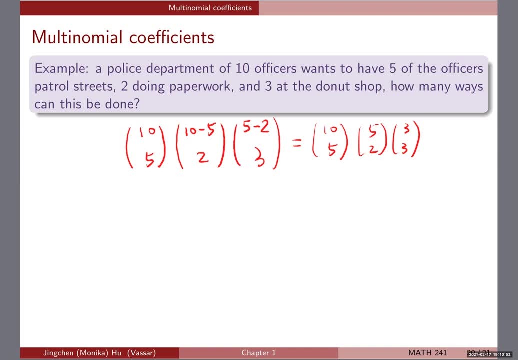 is: we know one property right And choose. n is always one, so that goes away, okay? Well, it's one. so it's straightforward And let me show you, once we have broken it down into using the 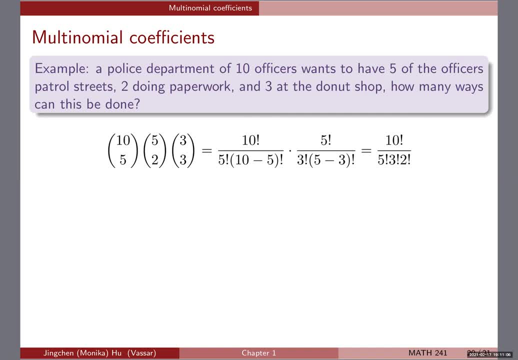 well, now, this is using the combination definition, the choose function, and break it into all of the factorial notation, and we start to see that we're able to cancel out certain things. Okay, so this five factorial can cancel out with this five factorial. and then this is actually: 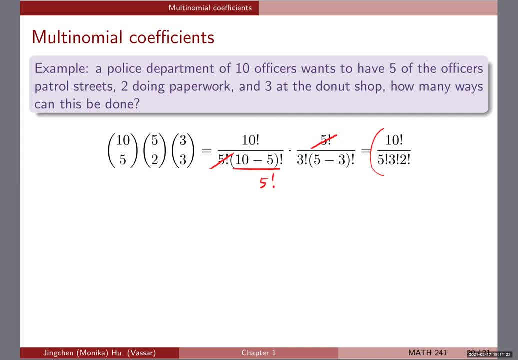 another five factorial. So in the end we have this 10 factorial divided by five factorial times three factorial times two factorial. okay, So this, if you remember one of the permutation scenarios that we talked about, right, If we have n objects and we have all of them, 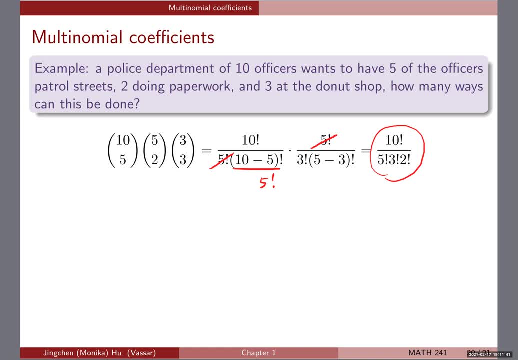 remember, some of them in one group, some of them in the other group, and then the total number of permutation is one, and then the total number of permutation is one and then the total number of permutations in that kind of scenario actually is the same. result is n factorial divided by n. 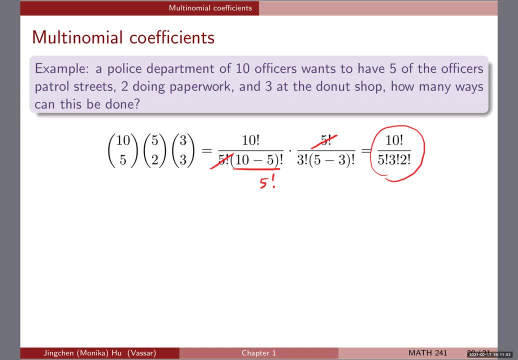 one factorial and two factorial, et cetera, et cetera. okay, However, here, notice that we're not doing permutation. okay, We are not caring about the order. as we know, back then, permutation always cares about the order. Now, we're really just like grouping. right, We're grouping. 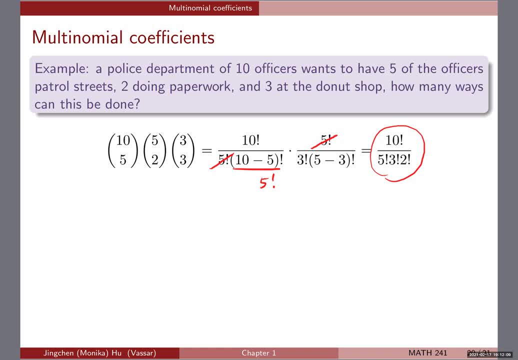 10 objects or 10 officers into three different groups? okay, And we're trying to figure out the number of ways to do that. okay, So from here we're able to introduce the binomial- sorry, multinomial- coefficient. okay, So generically, let's look at the question. 10 officers- they're. 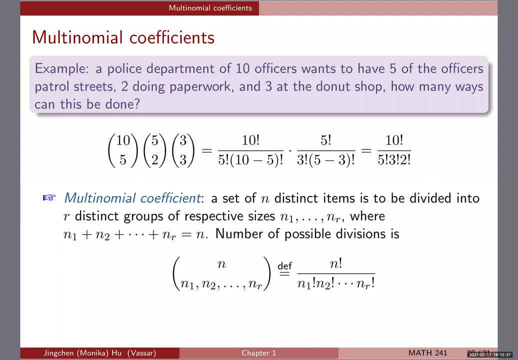 all different from each other. okay, So we have a set of n distinct or different items or objects and we want to divide them into r distinct groups. okay, So in this example we have one, three groups right: One for patrolling street, one for paperwork and then one for donut shop. 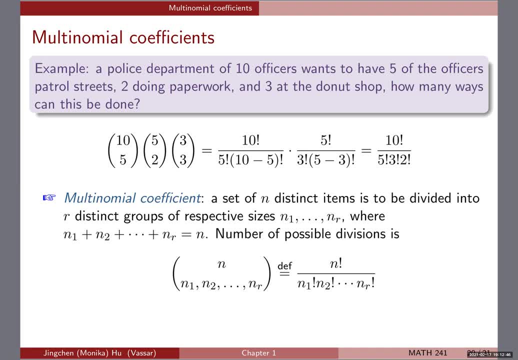 right. So we have three distinct groups of respective sizes and we're given what the sizes are: right: Five for the first, two for the second and three for the last. So the number of possible divisions, which is actually a multinomial coefficient in this case, is defined well. 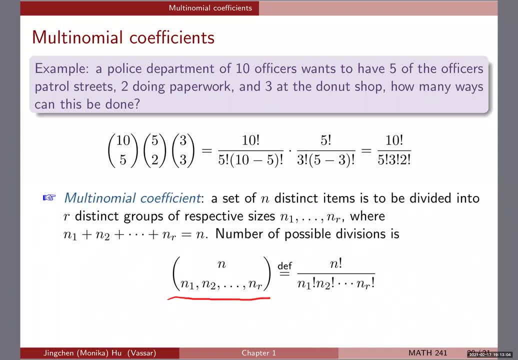 notation-wise, we have this really tall and wide choose function. You have the total number, the number of distinct items, at the top, and then you just list all of the group sizes, okay, the bottom, with comma separating them, And, by definition, well, this is the number of possible. 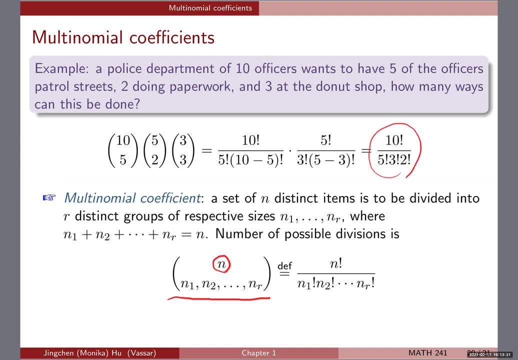 divisions that we have just seen. Well, you can cancel out all of the intermediate terms that you can imagine and then you are reduced to n factorial, divided by the product of all of the size factorials. okay, So, like I said before, you can always start with a particular example to 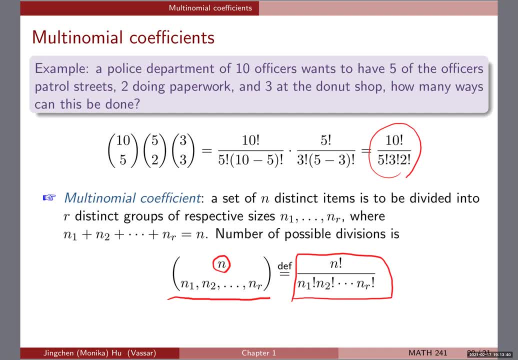 understand why that is the case, but then from this particular example, we have seen those constellations and you can see that if you have so many, so many items in between, they're going to get canceled out like one by one. So eventually, 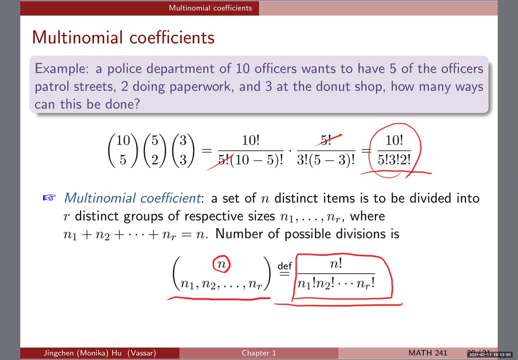 you're always going to get n factorial right divided by the factorial of each of the sizes that we're doing okay. So this is multinomial coefficients, okay, And what we're doing is we're trying to divide n distinct items into our distinct groups, and we also know the sizes for 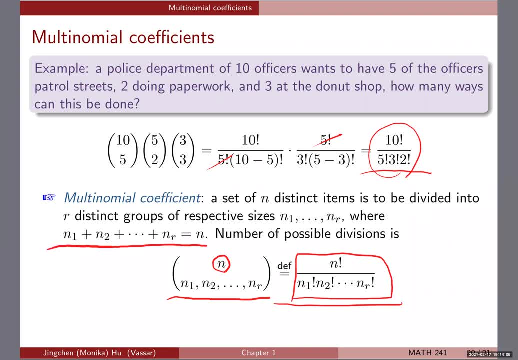 each group And, in particular, I should highlight that, well, the size, all of the size, should add up together to the total number of items you have. Okay, so, multinomial coefficient, and then, well, this is like I said, you can really. 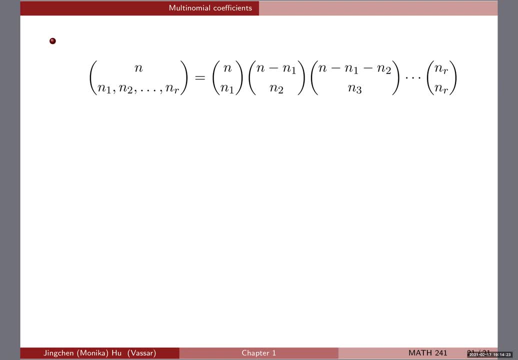 if you go back to the officer examples, we know that, well, we're really choosing one group at a time, right, And then for each case you're subtracting whatever you have chosen from the total that you'll be able to choose from for the next step of the choose function. So that's why. 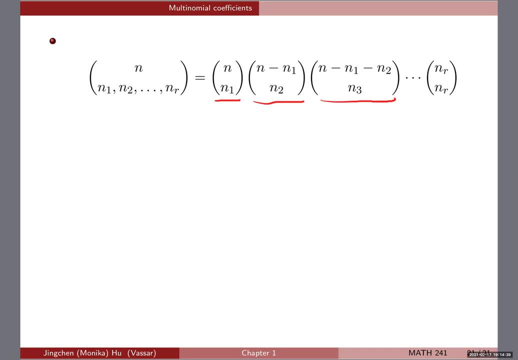 later on you will see that many of them get canceled out and then you get the final result is what we have seen before: okay And well. multinomial is. what we were talking about earlier is a generalization of the binomial. 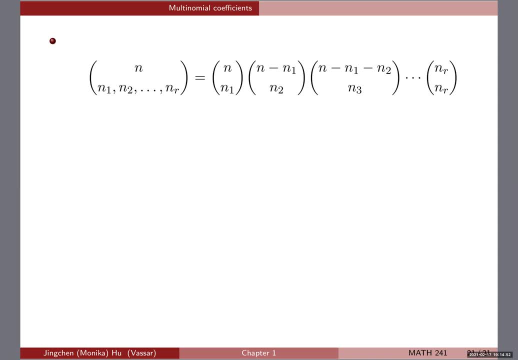 okay, Binomial, you have two outcomes. Here you have more than two. So if r, which is the number of groups that we're talking about, is two, this binomial, this multinomial coefficient, actually reduces to the binomial coefficient. okay, It's just the choose function itself, okay. So this: 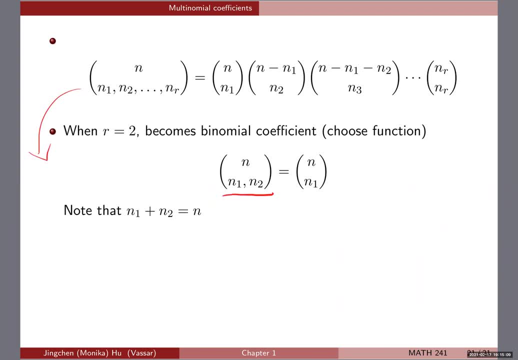 one. as we know, if we follow the definition from before, this will be n, sorry n. choose n1, right, And then the remaining is n minus n1. choose n2, okay, But this whole thing we know is: 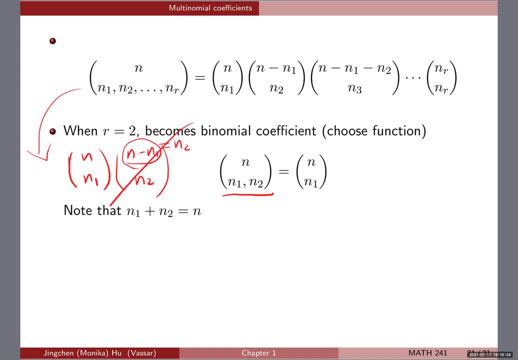 n2.. So n2, choose. n2 got canceled out, It's one. So well, it is reduced, as we can see, to the binomial coefficient. And don't forget that the sum of the n1 and n2 needs to be n. okay. 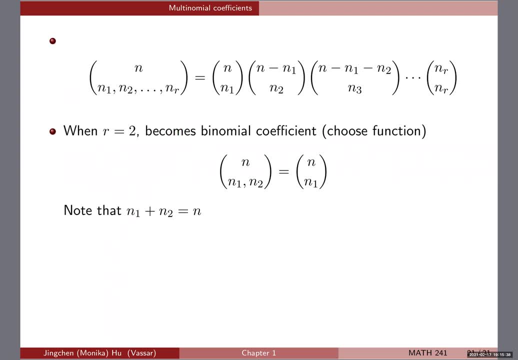 And, lastly, we have binomial theorem, right, So we also have a multinomial theorem. It will be a less, I guess I should say less- intuitive and more challenging to understand. why exactly the case, But just to give you an example of why this could work. So remember the license plate example. 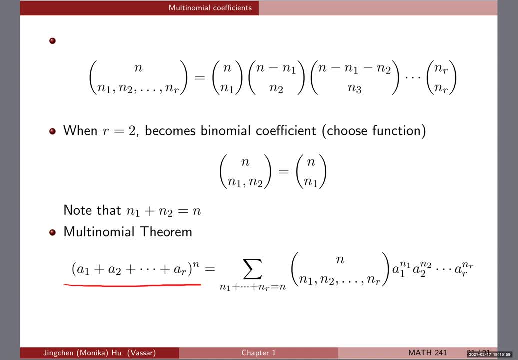 we use for introducing the binomial theorem. binomial theorem: right, We have A plus B to the power of N, okay, And we know that A is the number of letters you can choose from, B is the number of numbers you can choose from, and then you have integers that you can do. So the left-hand. 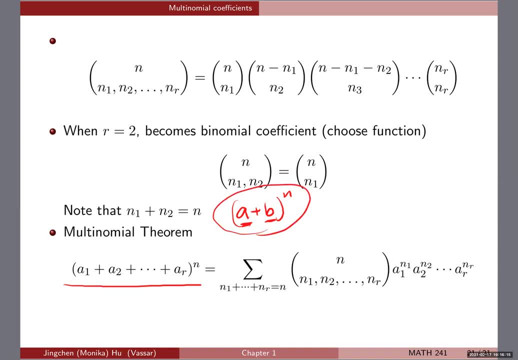 side. back then, what we're showing over here is the number of distinct license plates you're able to have, And the right-hand side. if you remember, we're breaking it down into each case, each of the cases where we're considering exactly K number of letters in that case. So now generalize it to the 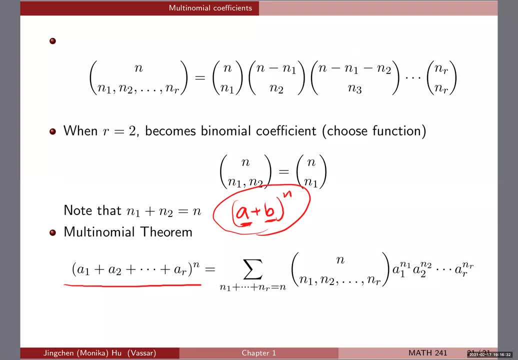 multinomial theorem. Maybe one way we can think about it is that: well, instead of only having two choices for the license plate for each digit, let's just say we can choose from 26 capital letters. Okay, And let's just say we can choose from 26 small letters, And then we can also choose from. 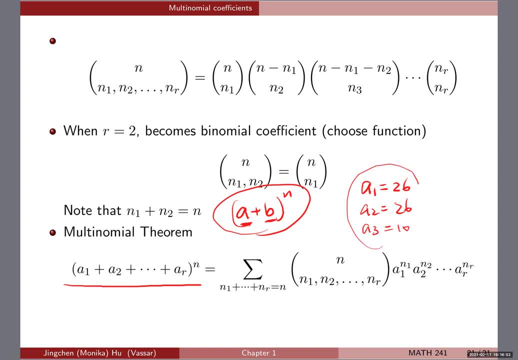 10 digits. Okay, So okay, This is the case, right, That? well, in addition to capital letters and the numbers, we can also choose small letters. So the left-hand side, as you could imagine, now it's going to be 26 plus 26 plus 10, to the power of N, which is the number of digits. 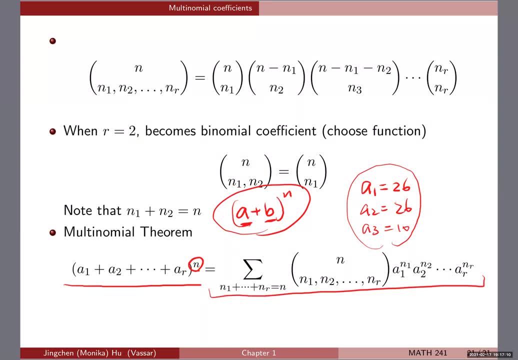 The right-hand side, of course. well, again, it's more, more involved, as what we're talking about, as before. But again, as you can see that the summation is again looking at the sum, well, in our case we have three groups, So R equals to: 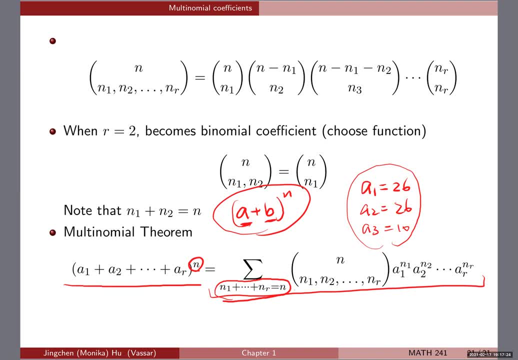 three, right? So we're looking at the sum and then you can think about. each of the terms in the sum will be a exact number of combinations of the like, say the exact like N1 and N2 and Nr. number of um. well, in this case, let me just say out loud: 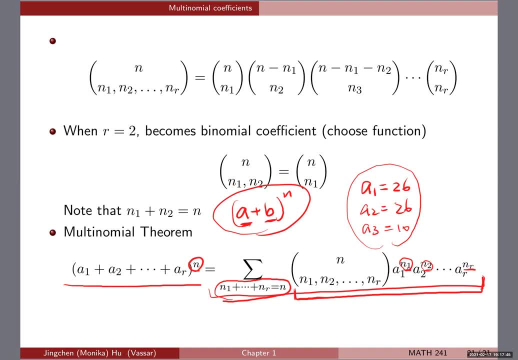 N1 will be the number of capital letters. right N2 will be the number of small letters, And then we only have an N3, which will be the number of um digits. uh, like letter, sorry, the number of. 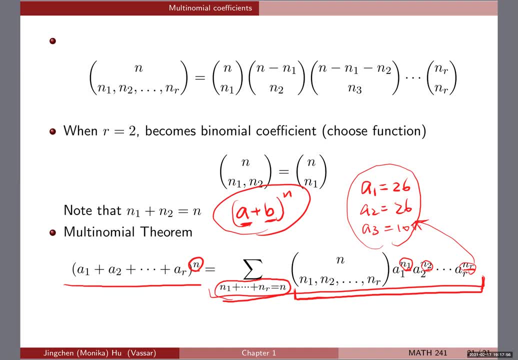 numbers, uh, to be used in the digits. So well, and then we have this. if you remember the multinomial coefficient, that's a sequence of choose functions. So the right-hand side, in sum, is trying to also show you that. well, the total number of license plates can also be deduced by: 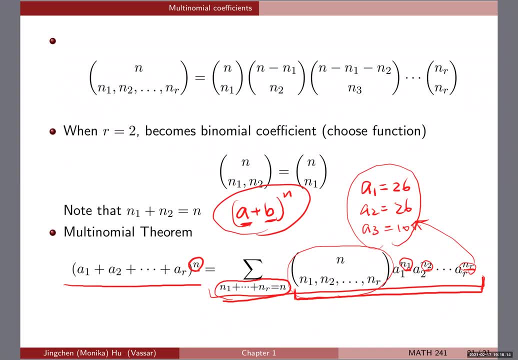 uh, counting, uh, a particular combination of the three numbers that you're able to come up with. add up to N, And then each of those is a choose function. times those powers together. Okay, So not surprisingly, like what we have seen before, if R equals to two, 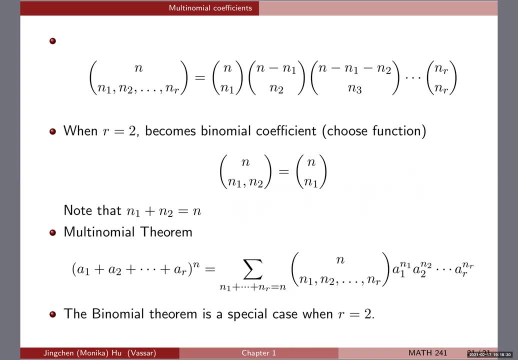 this is a binomial theorem, So binomial theorem is a special case of the multinomial theorem. Okay, So multinomial theorem and then the coefficient overall. uh, they're really useful when you are dealing with more than two groups, like, oh yeah, more than two groups.